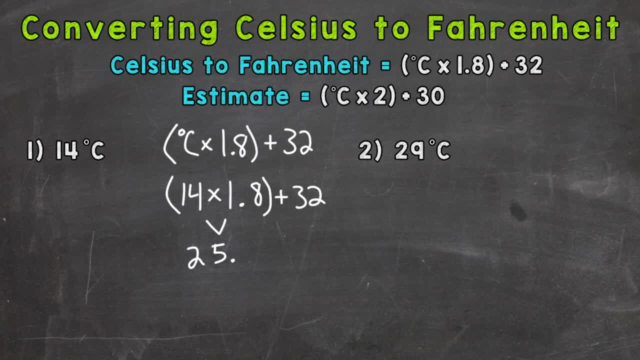 So you can either do that by hand or punch that into a calculator. Either way: 25 and 2 tenths, Then we add 32.. So 25 and 2 tenths Plus 32 is going to give us an answer of 57 and 2 tenths degrees Fahrenheit. 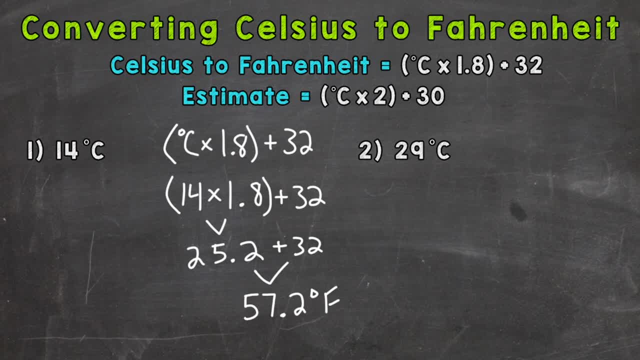 So 14 degrees Celsius equals 57 and 2 tenths degrees Fahrenheit. Now, as far as estimation, we can use degrees Celsius times 2 plus 30. So I rounded the numbers in the original formula to simpler numbers to work with As far as mental math and coming up with an approximate or close conversion. 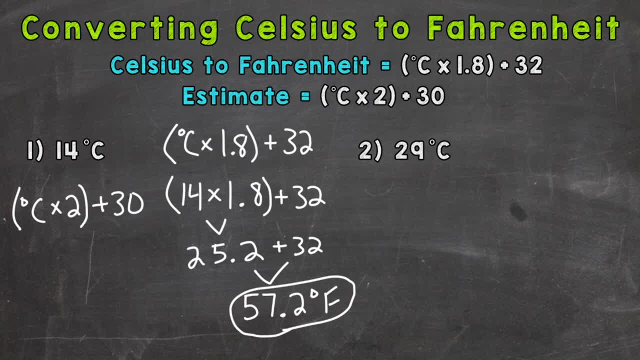 So, for example, number 1,, we can do 14 degrees Celsius times 2,, which is 28 plus 30, is 58. So this formula would give us an estimation of 58 degrees Fahrenheit, which you can see is pretty close to the actual conversion. 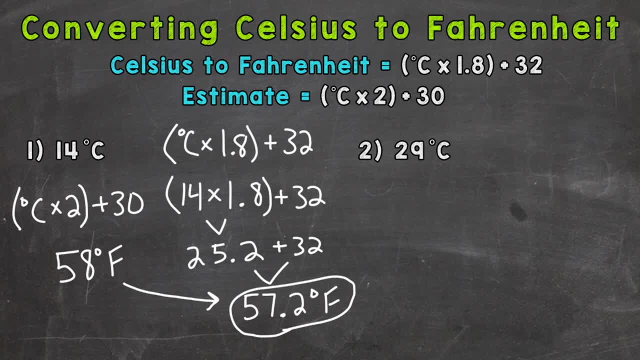 So that would give us a good estimate there. On to number 2, where we have 29 degrees Celsius. So let's write out our formula: Degrees Celsius times 1 and 8 tenths plus 32.. So we plug in what we're given and what we want to convert. 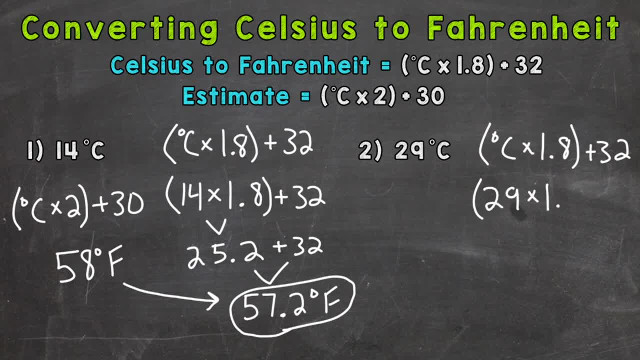 which is 29 degrees Celsius times 1 and 8 tenths plus 32.. So 29 times 1 and 8 tenths is going to give us an answer of 52. And 2 tenths plus 32, and our conversion is going to be 84 and 2 tenths, and that's degrees Fahrenheit. 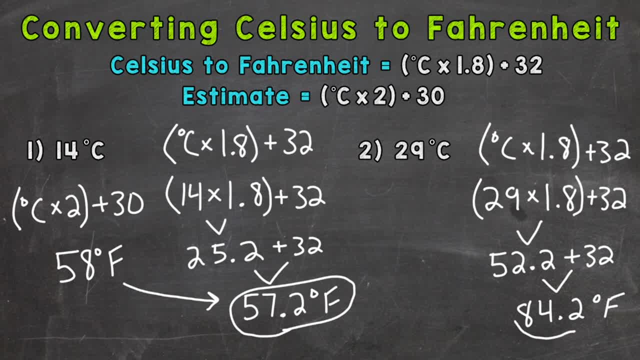 So 29 degrees Celsius equals 84 and 2 tenths degrees Fahrenheit. Now as far as the estimation for number 2, we are going to use the formula right here: Degrees Celsius times 2 plus 8 tenths. So 29 times 2 is 58, plus 30 gives us an estimate of 88 degrees Fahrenheit.